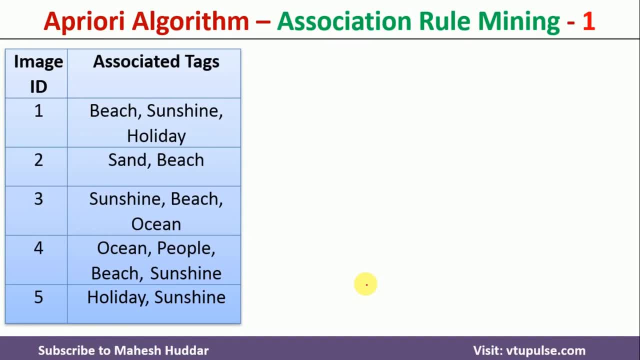 Actually, it has five image IDs and there are associated tags in this case. Now we need to apply a priori algorithm to discover the strong association rules, given the minimum support of 40% and minimum confidence of 70% in this case, To generate the strong association. 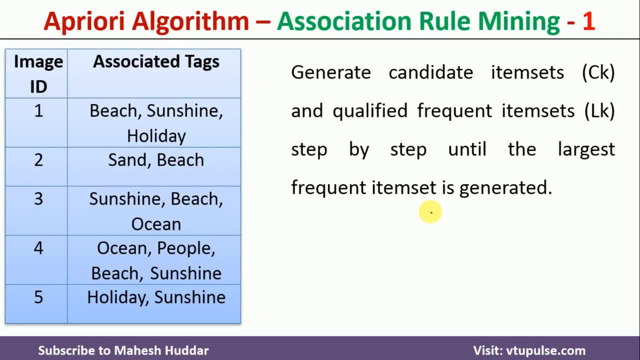 rules. first we need to generate the item sets and then we need to find the qualified frequent item sets based on the minimum support. Once you get the largest frequent item set then we can start building the association rules here. So first I will try to explain how can you get the 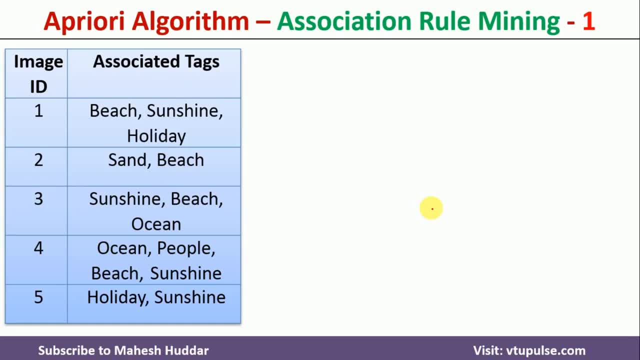 frequent item sets step by step. In the first step we need to generate or we need to get the support count for individual item sets. that is one item set. So in this case the beach holiday was seen and so on. are the one item sets The number of times beach appears? 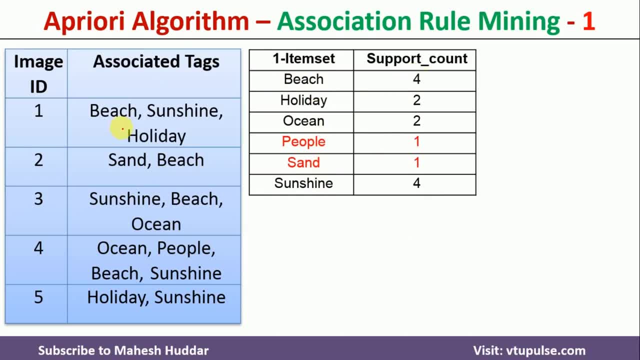 we need to count and then we need to write in the second column. So if we see here, beach appears one, two, three and four times. So that is what I have written here. Similarly, holiday holiday appears once here and then the holiday appears one more year. So I have 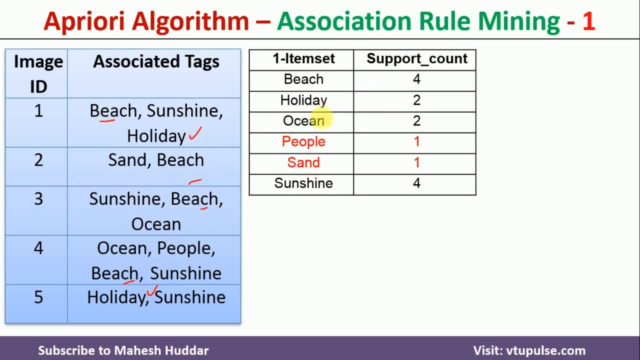 written two in this case. Similarly, I have to write the frequency of one item set in this case. Once I write this particular support count of one item set, Now we need to select the qualified item sets, in this case as a one frequent item set. So in this case we: 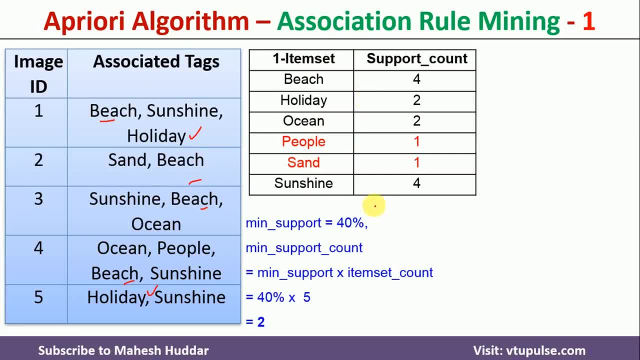 have one frequent item sets. For that reason we need to check what is the minimum support given to us. The minimum support given to us is 40%, So the minimum support count expected is equal to minimum support multiplied by item set count. So minimum support is 40%. 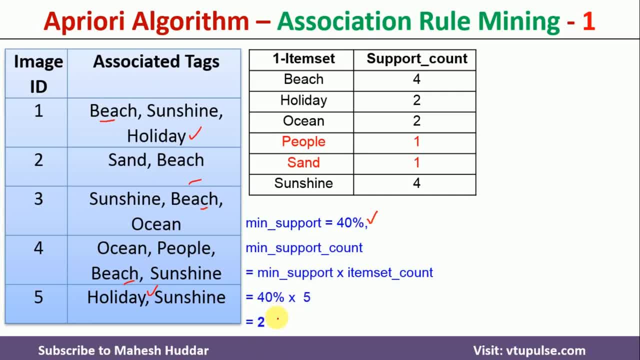 multiplied by five, that is equal to 200%, which is equal to two in this case. So the minimum support is two. So if you have the minimum support count of two, the meaning is that item set is a frequent item set. So in this case I have written beach, holiday, ocean and sunshine as 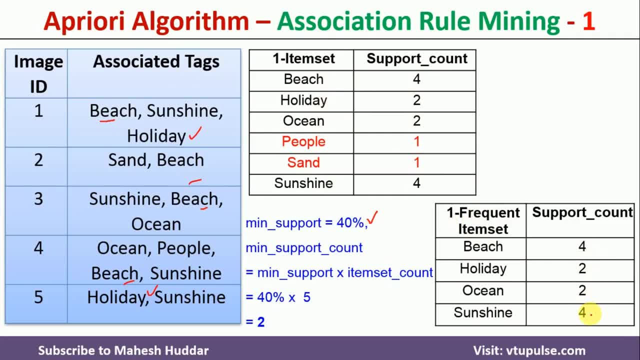 a one frequent item set because the minimum support count is two or more in this case. So this is how actually you can calculate one frequent item set: The same process we apply to calculate the two frequent item sets, For that first we need to find the two item. 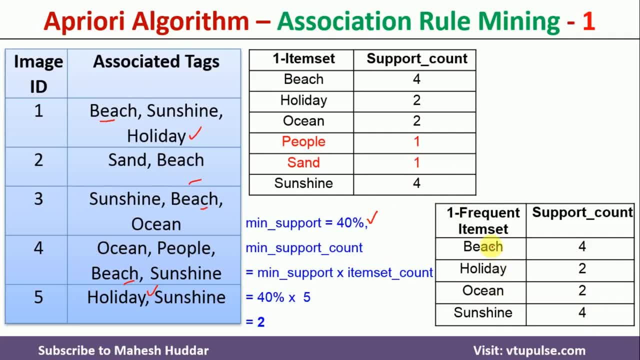 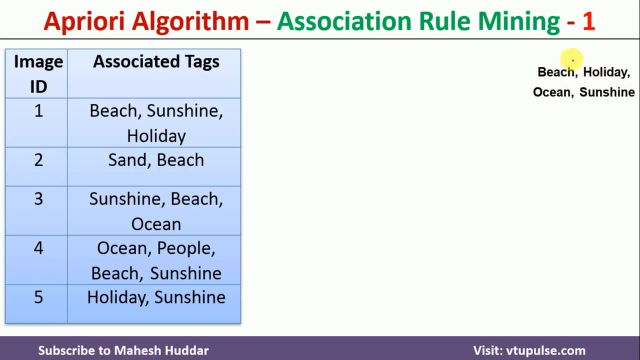 sets. To generate two item sets, we need to know the distinct one frequent item sets. The distinct one frequent item sets are beach, holiday, ocean and sunshine here. So that is what I have written here. Now I have to take two at a time. that is, beach, holiday, beach. 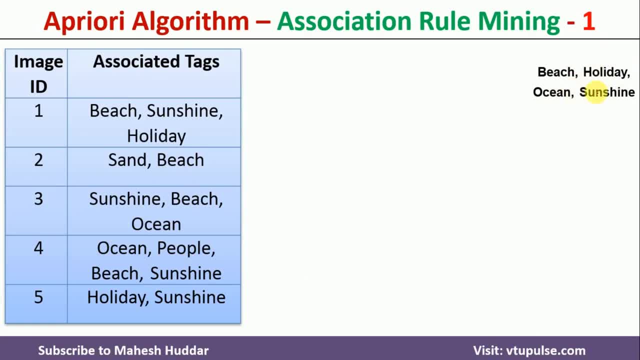 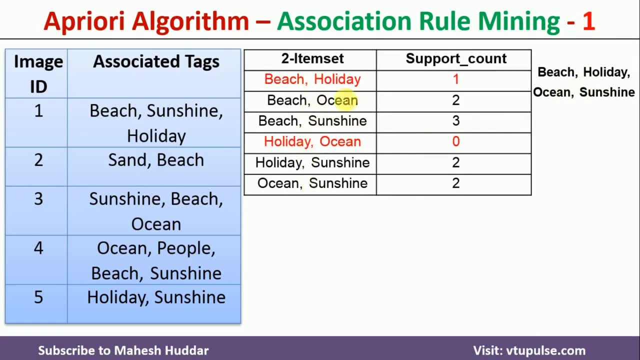 ocean, beach sunshine holiday. ocean holiday, sunshine, ocean sunshine. So these are the different combinations are there? I have written all those particular combinations. Now we need to count the support count for these items. beach and holiday: beach and holiday appears once here And if you see anywhere, we don't have any beach and holiday in this particular associated. 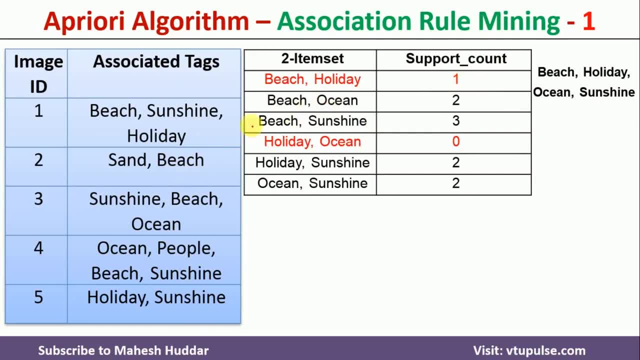 tags, So it appears only once. Beach and ocean. beach and ocean appears once here and beach and ocean appears one more time here, So it is appearing two times. Beach and sunshine, beach sunshine, beach sunshine and then beach sunshine. totally three, So it is appearing. 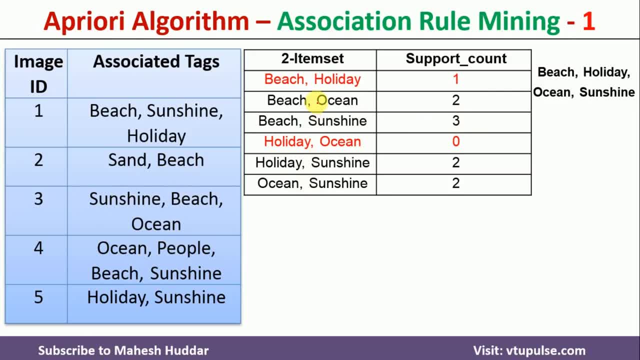 three times here. So similarly we need to count how many number of times the two item sets appears. So we have to take the two at a time and write it in the second column, Again the same process. The minimum support count expected is two. So the two item sets having two or more support. 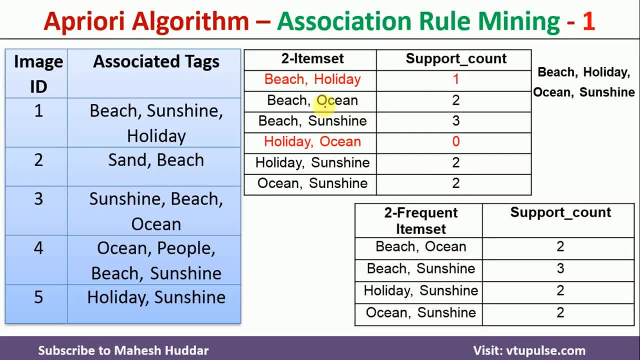 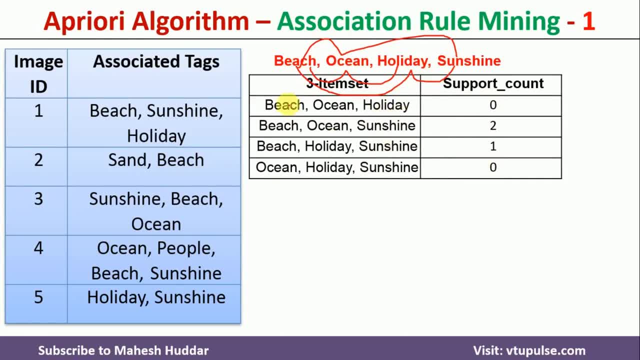 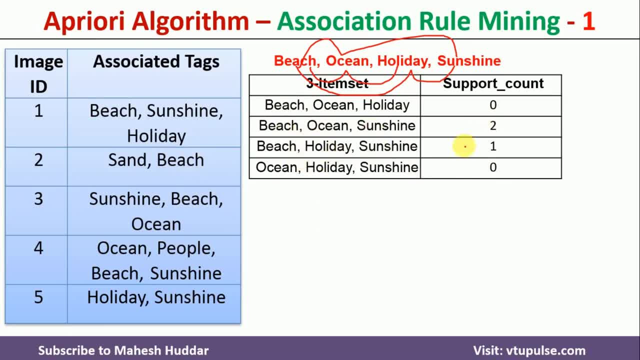 sunshine appears two times. beach holiday sunshine appears: one time ocean holiday sunshine appears: zero time. so that is what i have counted and written over here now, if you see this particular four possibilities out of that, this is second: one is only qualified frequent item set because it is having minimum support count of two in this case. so that is what i have written here now. 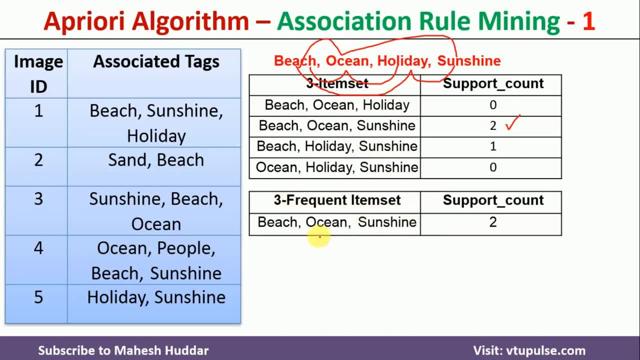 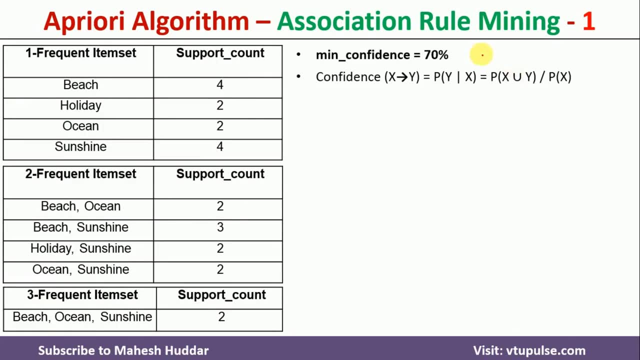 it is not possible for us to write four item sets as well as four frequent item sets, so we will stop here now. the next part is to find the strong association rules. so if you want to find the strong association rules, we have to use this particular formulae: the expected minimum. 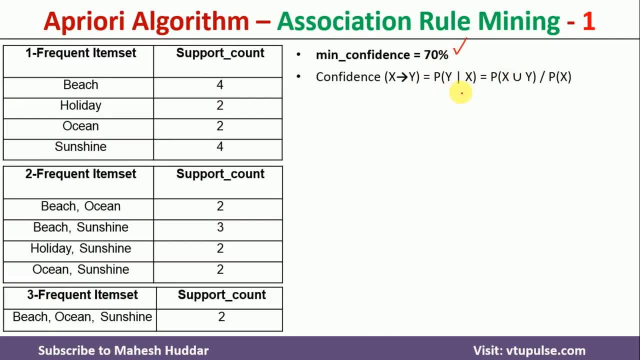 confidence is what? seventy percent? so how to get the strong association rules is: if you want to say that x tends to y is a strong association rule, it should have the minimum confidence of seventy percent. now the question is how to calculate the minimum confidence. the minimum confidence of x tends to y rule is the frequency that x and y both appears divided. 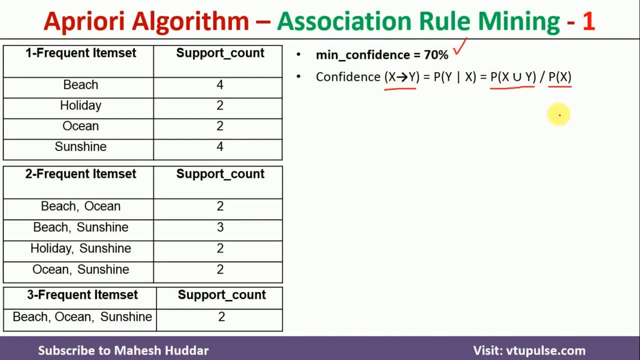 by the number of times, only x appears. so that is what we need to calculate. if it is seventy percent or more, it is a strong rule in this case. first and foremost thing, we will write: the frequency is zero. then the four common factors of the terms and essence, and therefore for every 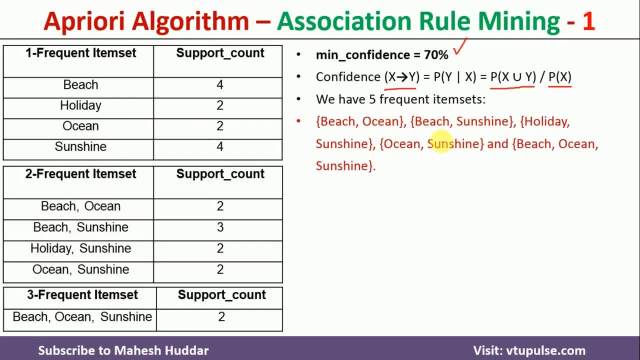 party will be a bound, he maximum confidence must be given and it is being set here. i will write the line or unique picks for each party and the fixed time are fixed, for example time. this is very important that whether x works or x also works. maybe x can also go foriko, f wrappedrijksch or c can also go forik, this one, but right here. 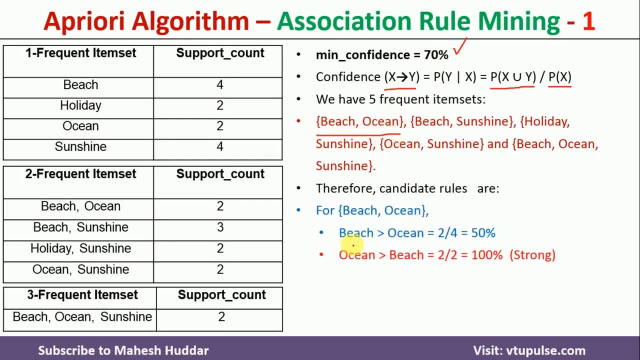 So if I consider beach ocean, there are two possibilities are there? either I can write beach ocean or ocean beach. If I write beach ocean, the number of times both appears- beach ocean appears two times here, divided by the number of times beach appears, number of time beach appears is 4. 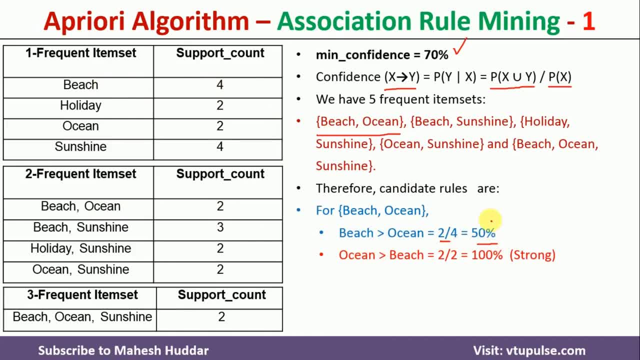 that is nothing but 2 by 4, which is equivalent to 50% here. This is not a strong rule because it is not greater than or equivalent to 70% here. Now I will consider the other side, that is, ocean beach. ocean beach both appears two times. 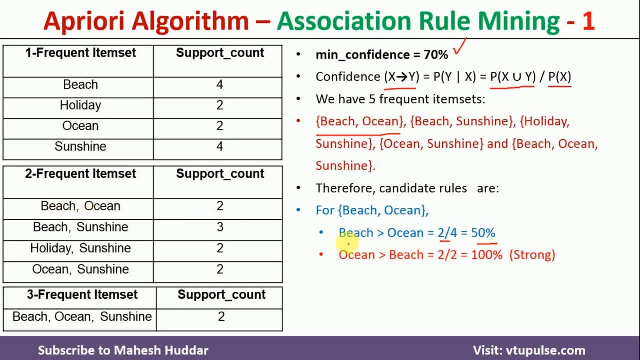 because ocean and beach appears two times. divided by how many number of times ocean appears, the ocean appears two times. so 2 by 2, which is equivalent to 100%. it is a strong rule in this case. Similarly, I will consider the second one, that is, beach sunshine, beach sunshine, beach sunshine. 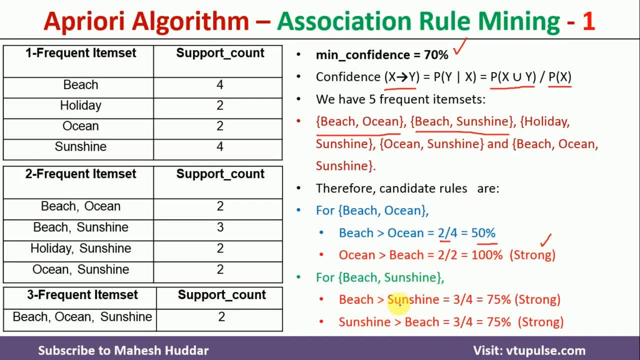 is the one rule and sunshine beach is another rule. So beach, sunshine both appears three times Divided by beach appears four times. so it is equivalent to 3 by 4, which is equivalent to 75%. because it is greater than 70%, it is a strong rule in this case. 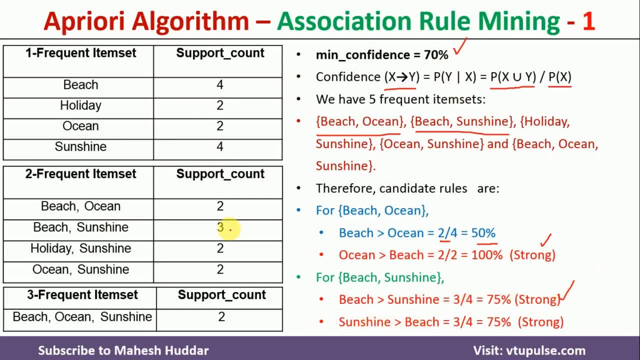 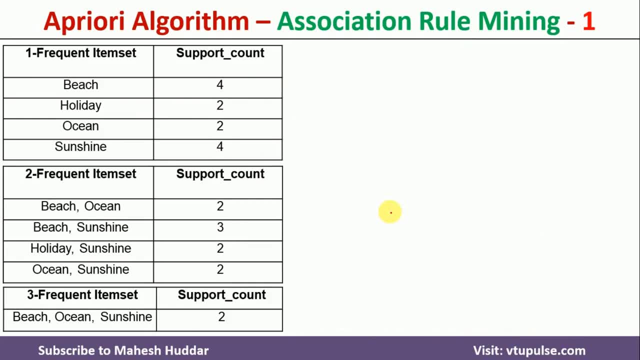 Similarly, suns beach and sunshine beach. sunshine beach appears three times, beach appears four times. so the meaning is it is 75%. again, it is a strong rule here. Now I will go with the next one. that is nothing but holiday sunshine. that is the next one. 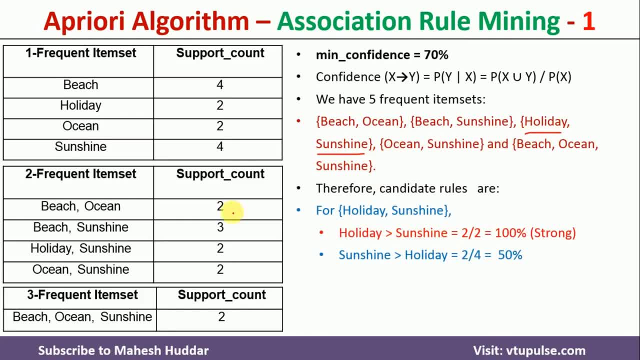 So holiday sunshine appears 2 times. I think holiday sunshine divided by holiday appears two times. so it is 2 by 200%, a strong rule. Sunshine holiday appears two times, but sunshine appears four times here. so 2 by 4, which is equivalent to 50%. that is not a strong rule here. 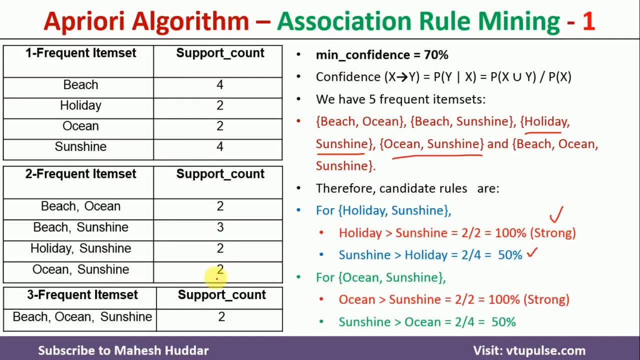 Next one is ocean sunshine. ocean sunshine appears two times. divided by ocean, that is two times, so it is a strong rule. Ocean ocean appears two times, but sunshine appears four times here, so you can say that 2 by 4 is equivalent to 50%. it is not a strong rule. in this case, this is also not strong. 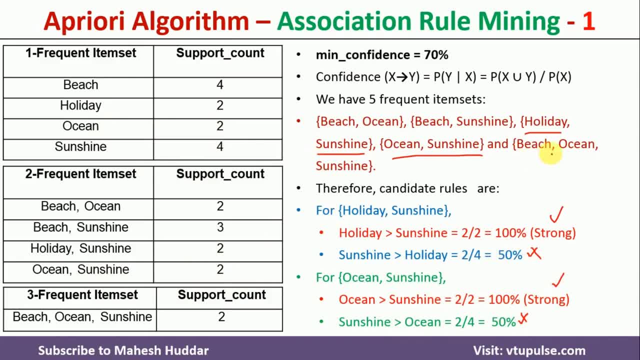 rule. this is also not a strong rule in this case. Coming back to the last one, that is, beach ocean, sunshine, we have multiple possibilities here, so I have to take these two: first, that is, beach, ocean and then sunshine, or you can write in any order, it is not a big issue. 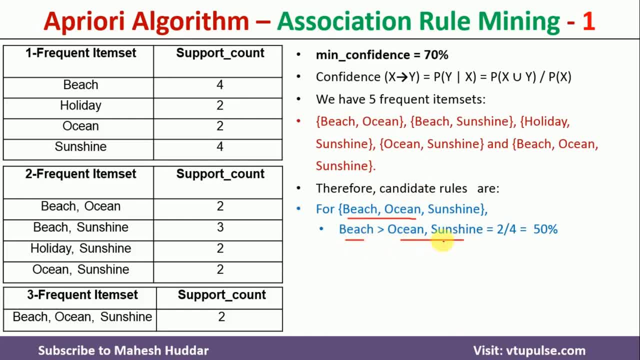 Beach, ocean sunshine- That is one possibility. how many number of times all three appears. all three appears. two times divided by beach, that is 4. so 2 by 4 is equivalent to 50%. it is not a strong rule. Next one is ocean sunshine beach. the other side of this one: two times all three appears. 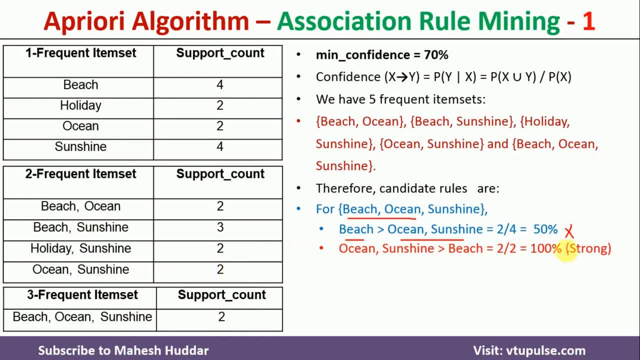 divided by ocean sunshine. ocean sunshine appear two times, so it is a strong rule here. Similarly, I have to consider ocean, this side, so ocean beach sunshine, and the other side, so all three appears two times, that is for sure. ocean appears two times here, so 2 by 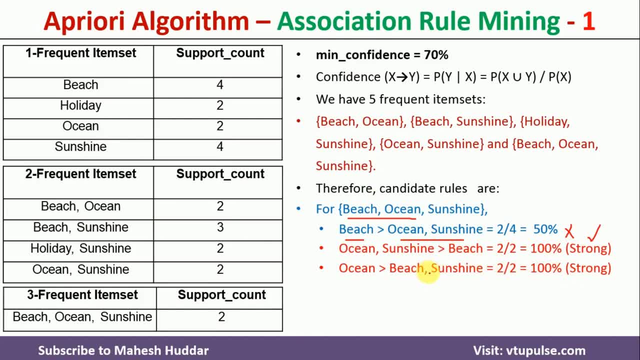 2 is equivalent to 100%. it is a strong rule. Now, beach, sunshine to ocean here, so all three appears two times. that is true beach and sunshine appears three times here. so 2 by 3 is equivalent to 67%. that is not a strong rule in this case. 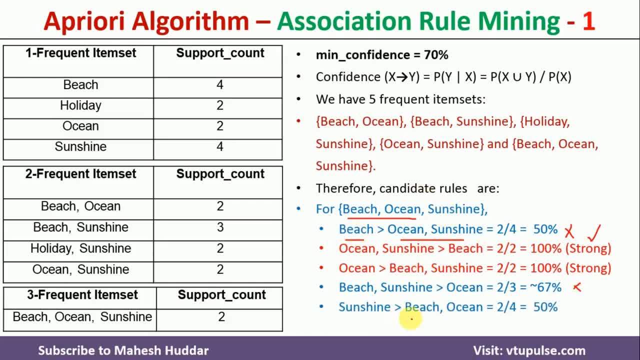 Now, coming back to the last one, sunshine, I have to take this side. So sunshine, beach, ocean, That is for sure Beach- all three appears two times. sunshine appears four times. so it is not a strong rule. The last one is beach ocean to sunshine: all three appears two times. beach ocean appears. 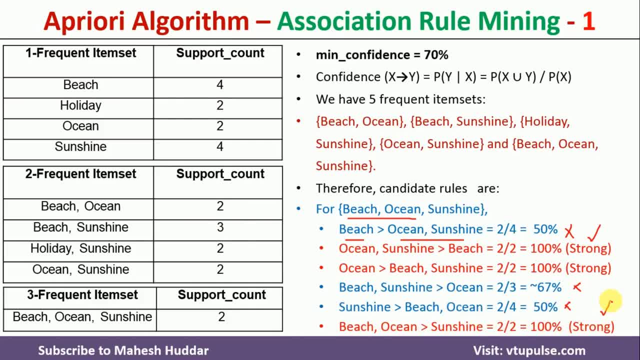 two times, so 2 by 2 is equivalent to 100%. that is a strong rule in this case. I hope you understood how can we generate frequent item sets, as well as the strong association rules, using a priory algorithm. If you like the video, do like and share with your friends. 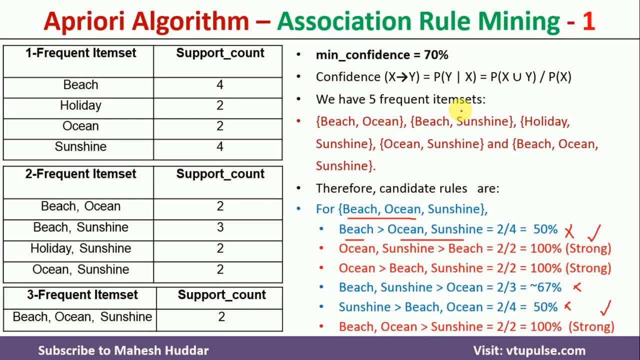 Press the subscribe button for more videos. press the bell icon for regular updates. Thank you for watching.